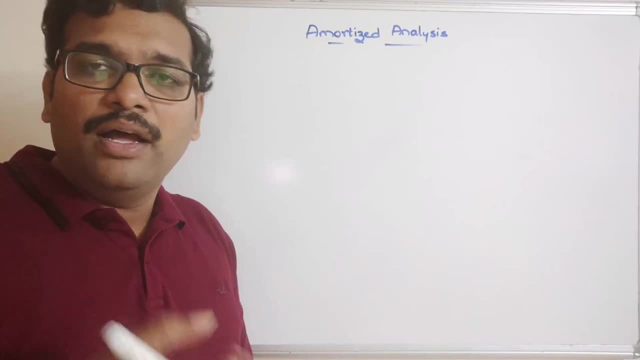 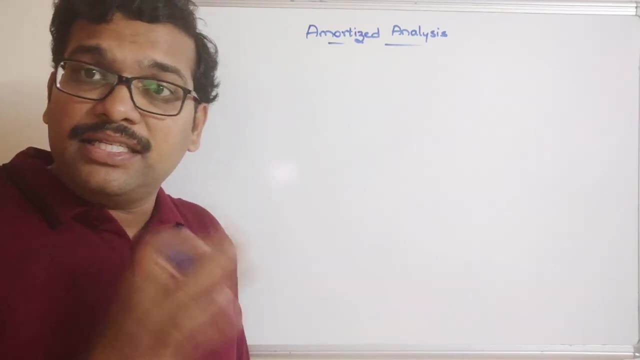 big theta and big omega notations which will give the worst case, best case and the average case complexity. So today we will see one more concept in algorithms. So today we will, And coming to this, amortized analysis. this is mainly used to analyze the average performance. 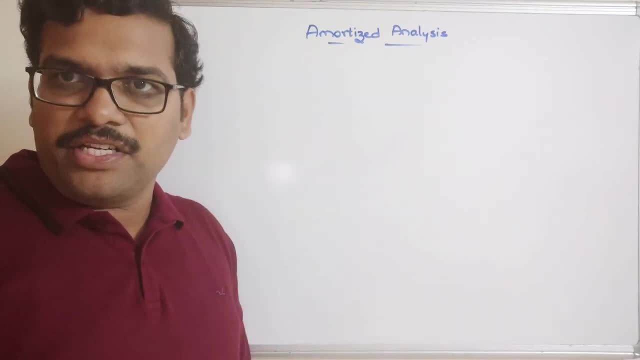 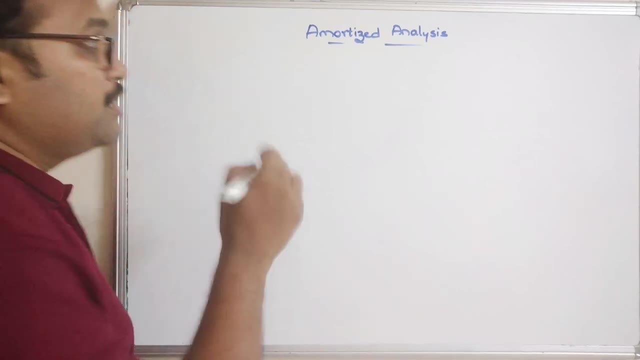 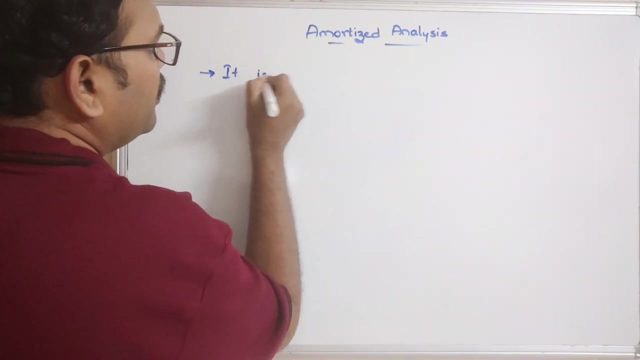 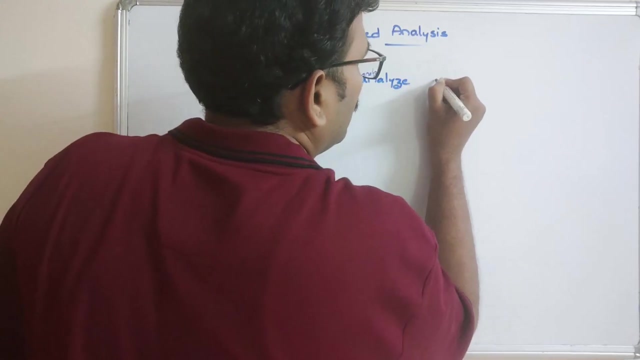 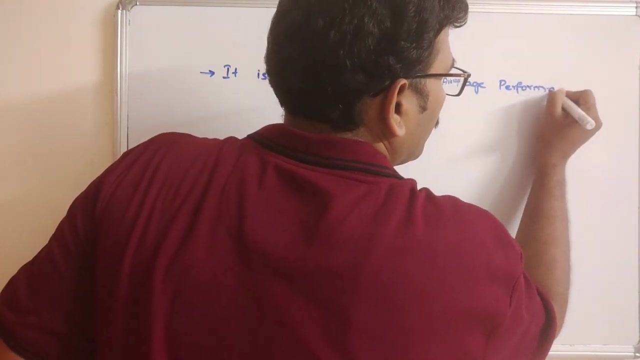 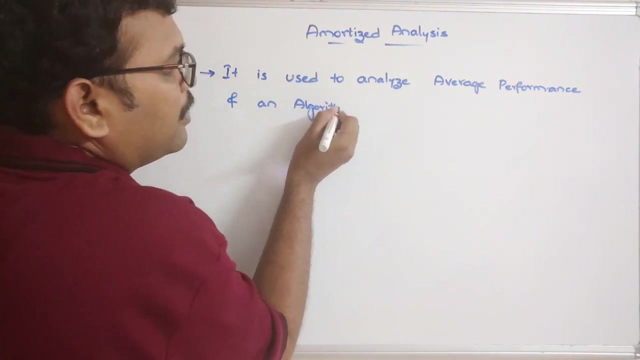 of the algorithm for a set of operations. So it is basically to find out the average time complexity. So that is also for a set of operations, So I will write here. it is used to analyze- analyze the average performance of an algorithm. This is most important. Next, for a set of operations: 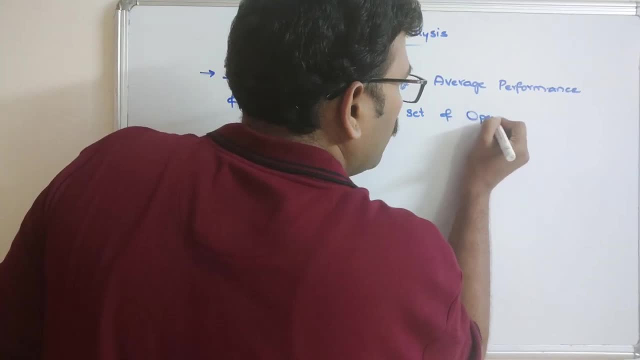 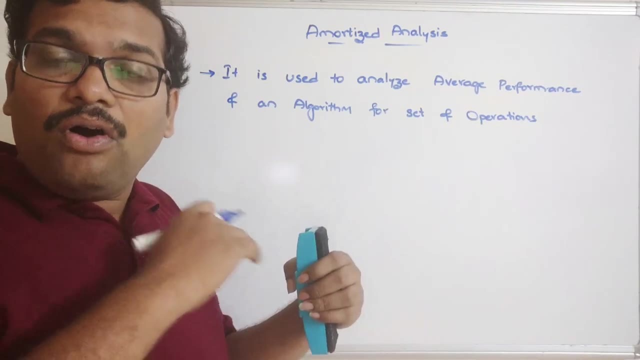 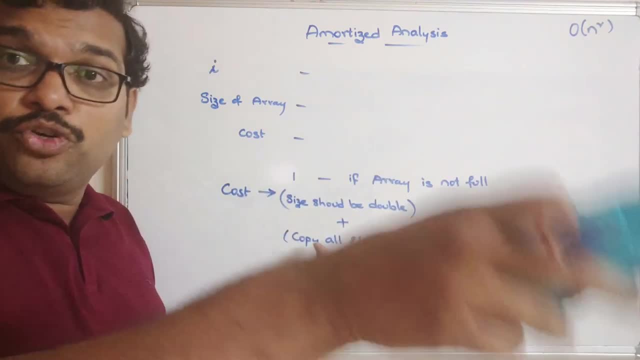 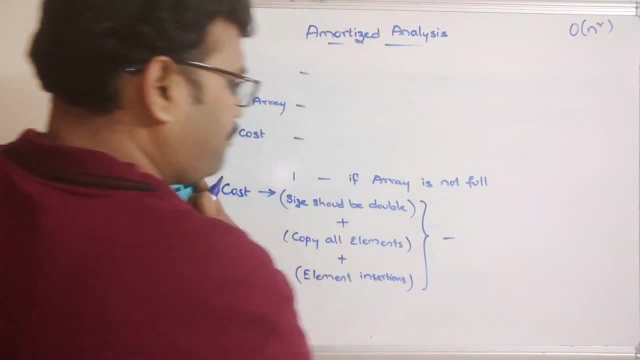 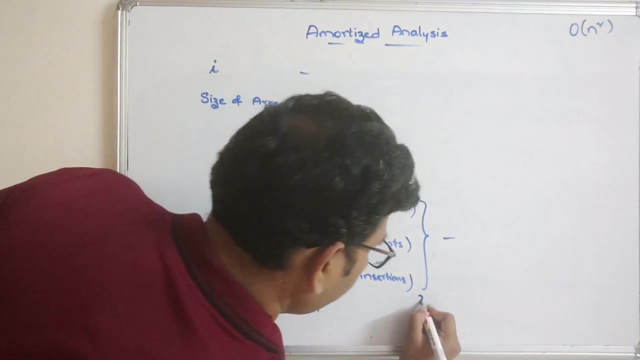 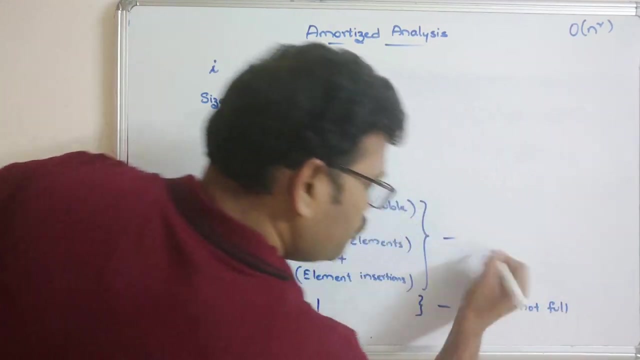 next step we have to copy all the elements, because every element should be in the continuous memory location, and then only we have to insert the element. so this happens. see, I'll write here, don't get confused. and it will be 1 if array is not full. this should be. happens if array is full. that means if the array is full. 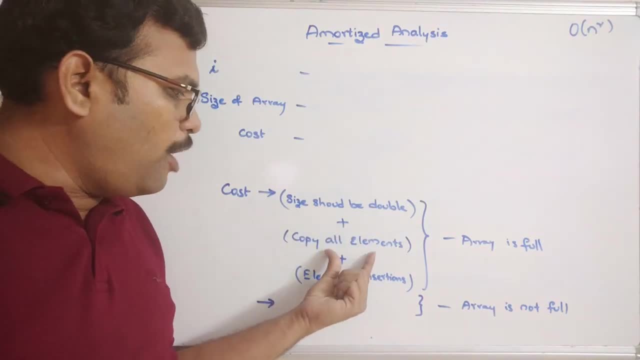 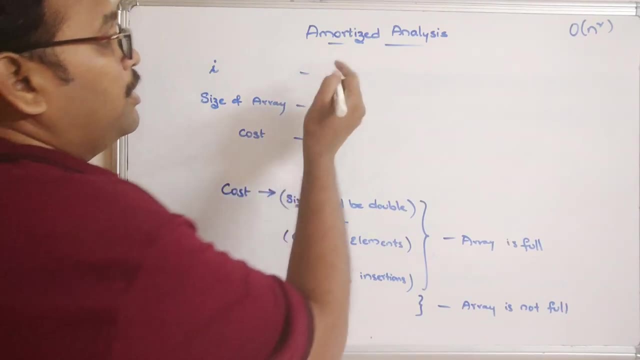 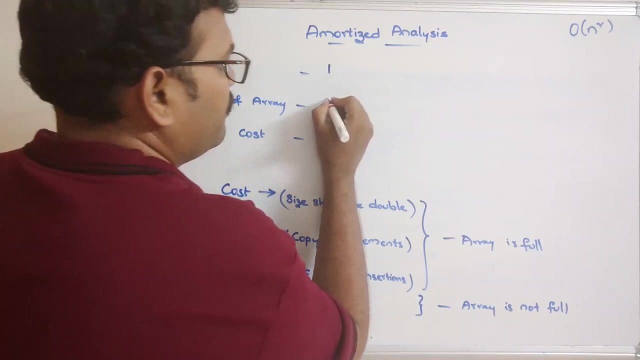 size should be double. that is the first one. copy all the elements. that the second one, elements insertion, will be the next one. now. so what happens if you are inserting one element and if the array size is 1? okay, so if the array size is 1, 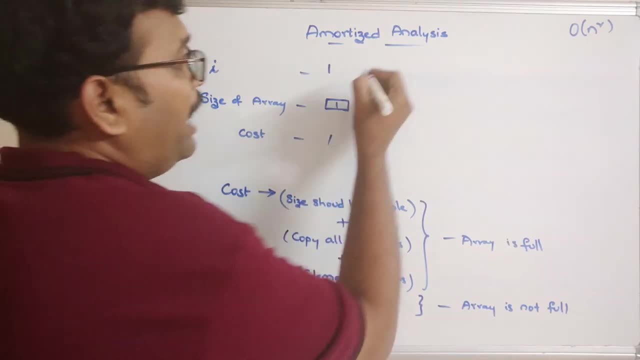 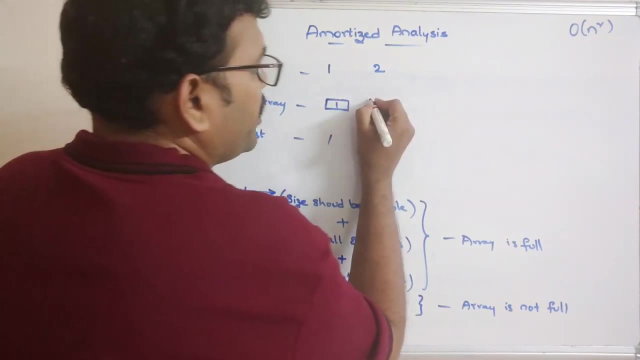 so simply, we can insert and the cost will be 1, and if you want to insert 2, the array size is 1, there is no empty. I mean the array is full. now it would be double. double means 2, so here it is 1 and here 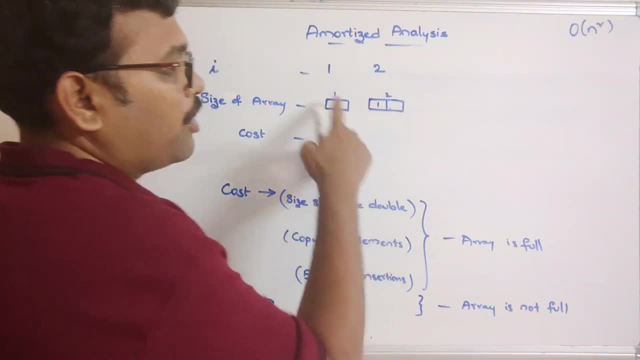 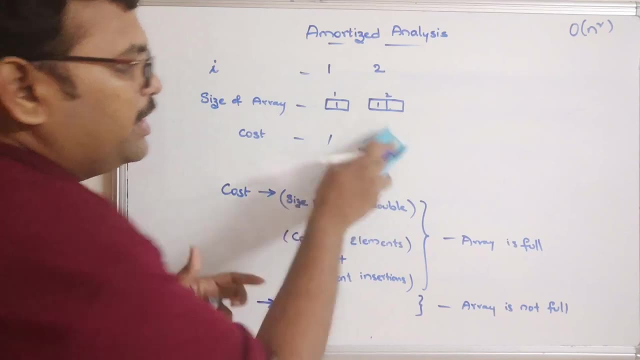 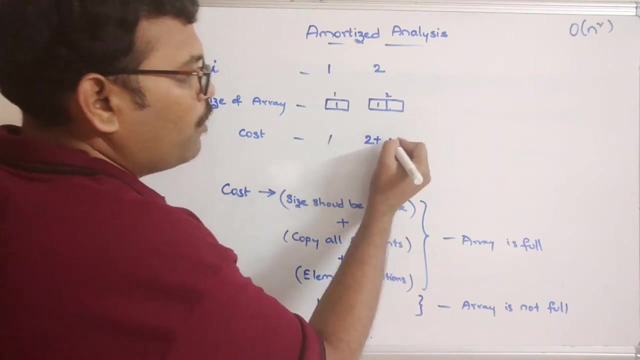 it is 2, so then insertion of copy the element. first we need to copy the element, so 1 plus how many element? so sorry, the first thing is double the size, so now the size of array 2, to next copy all the elements. one element will be copied and element of insertion one. 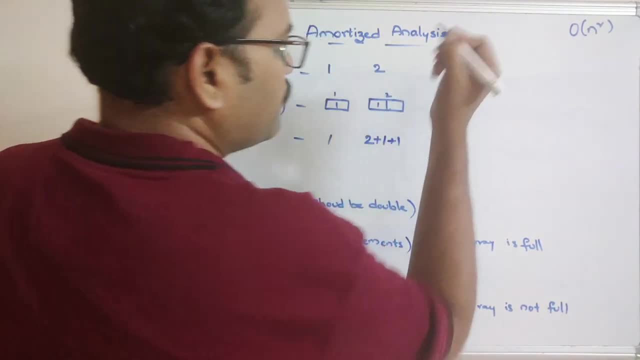 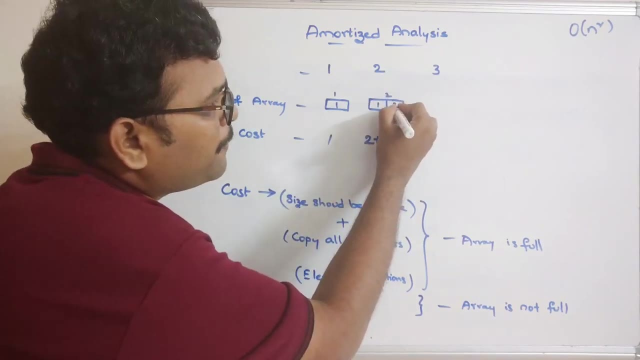 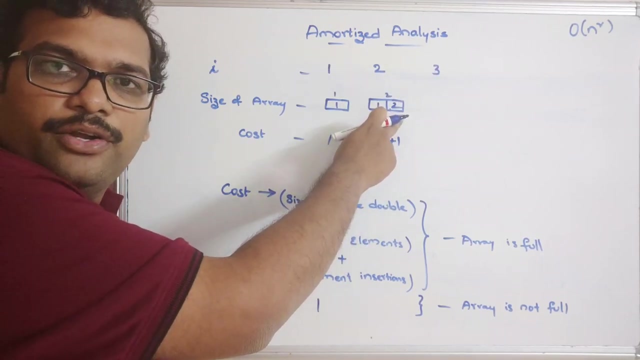 so the cost will be this one. and coming to the third insertion of the third one, so there is a blank. okay, so the array is not full, because, sorry, sorry, yes, so array is full. so array is full means third element can't be inserted into the size of array two. so then that should. 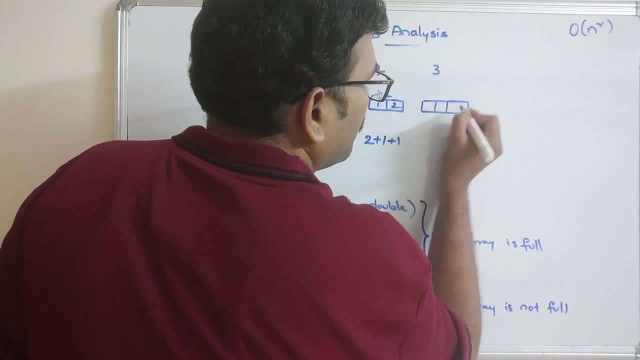 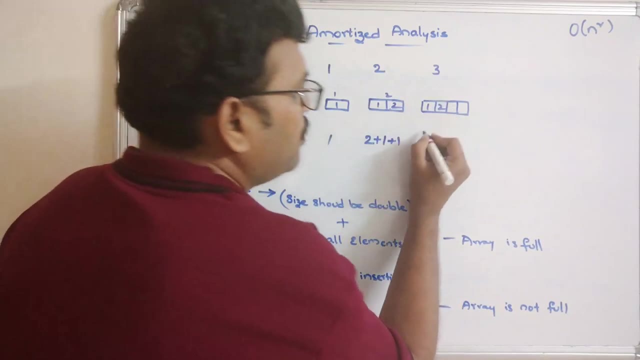 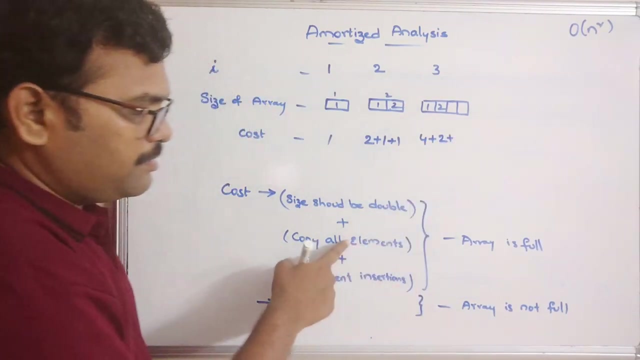 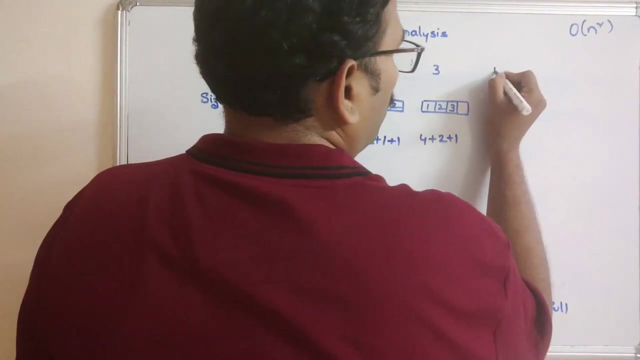 be increased, so one, two. and size should be increased. size should be double, so two. now it should be four. copy all elements. how many elements? two elements: two elements should be copied, plus element to be inserted: one. so here it is coming to the four element: four, so here. 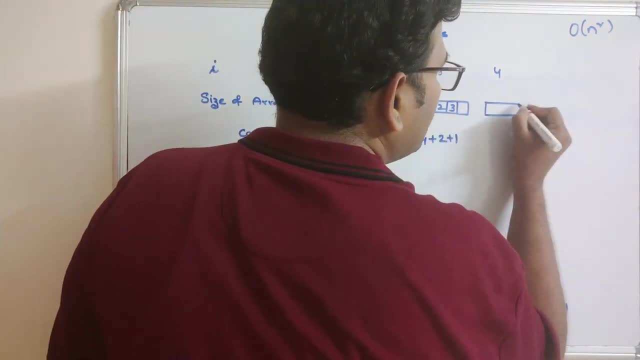 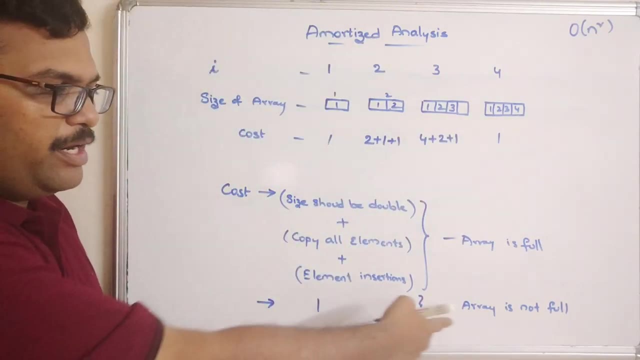 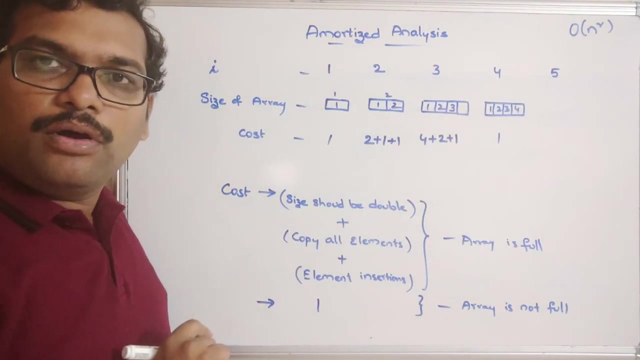 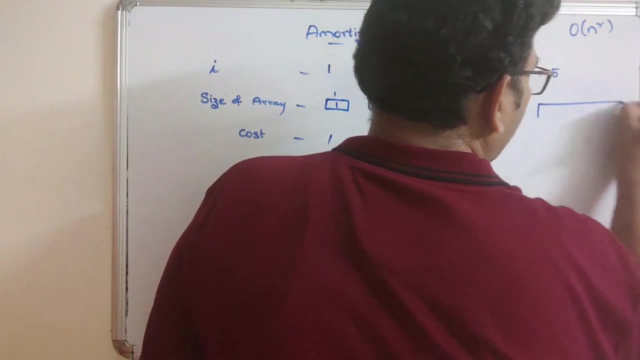 the array is not full, so obviously we can simply insert the element. so one, two, three, four, so the cost is one insertion of element. if array is not full, the cost is one, okay, and then fifth element. so there is no free space. so the array is completely full. what we have to do? size should be doubled. so now the size. 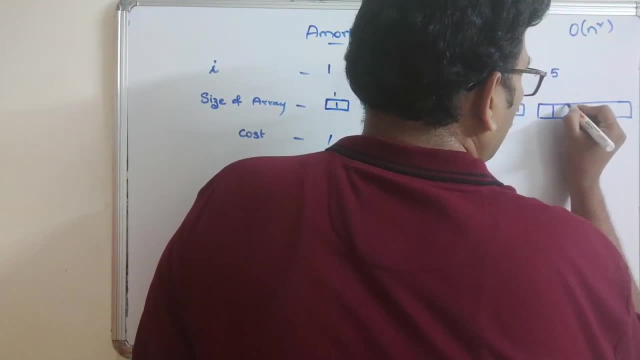 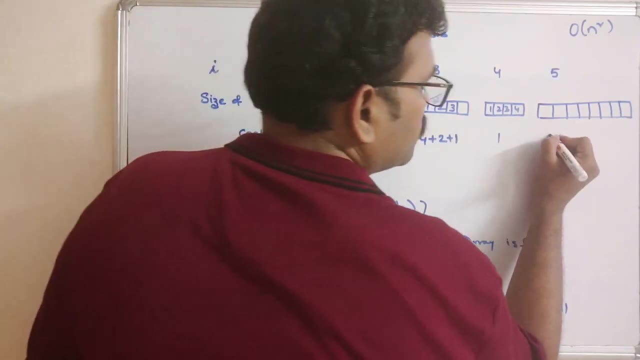 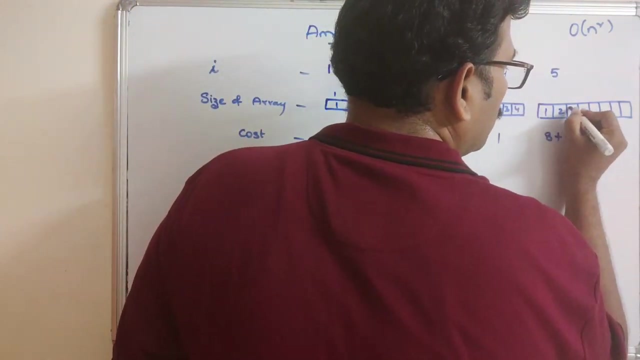 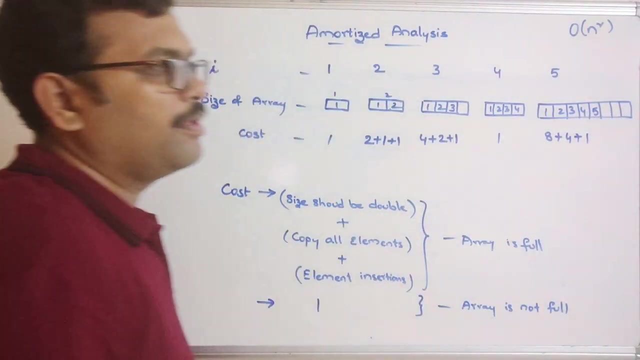 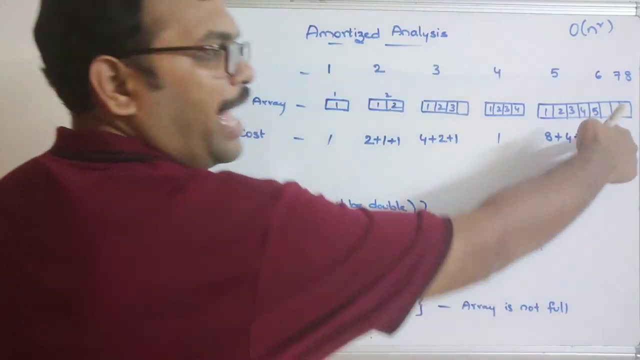 of array will be eight, right, so size should be doubled, so it will be eight plus copy all the elements. how many elements? four elements. four elements will be copied: one, two, three, four and one element should be inserted, one, so five, okay, and then for six, seven and eight. you can observe the array is not full. 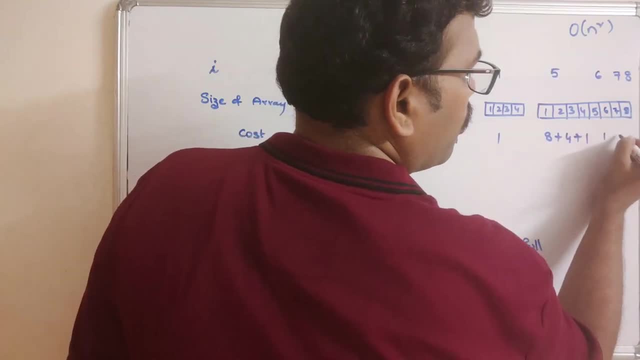 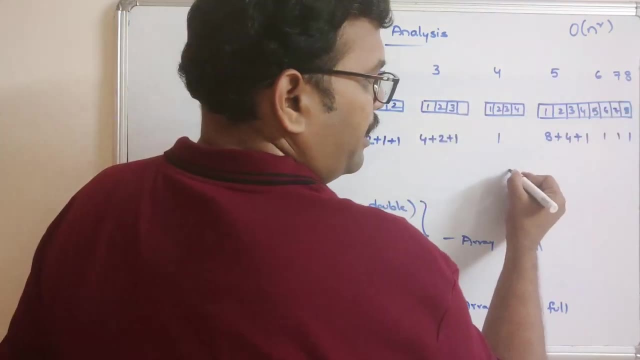 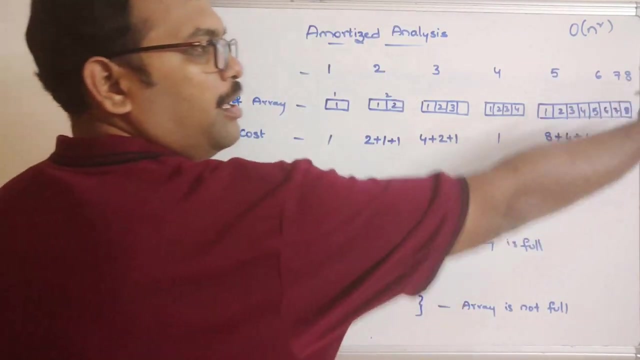 so obviously six, seven and eight, the cost will be one one, one right, because foot, and if, if it is again ninth element, ninth element, the cost will be how much? so the array is full. so it will be 16. first size should be double 16 plus copy all the elements. 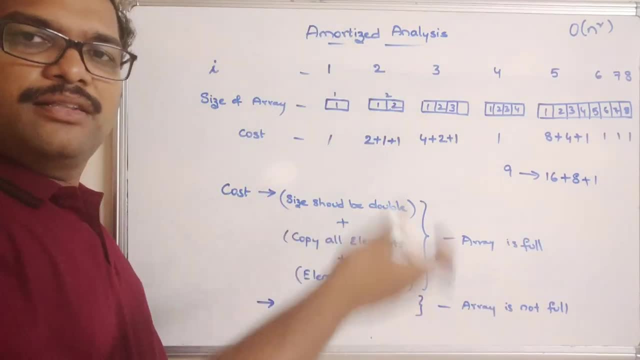 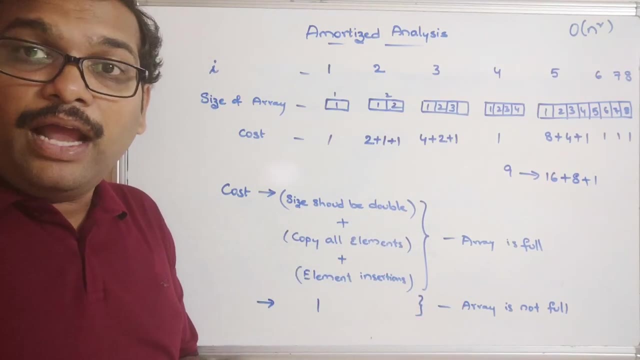 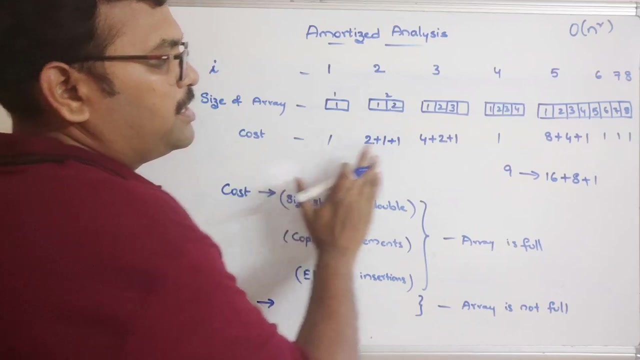 eight elements should be copied and plus one. so if you want to insert the nine elements, so that will be the cost. so like this, we have to analyze each and every step and what we have to do next we have to average the cost of all the operations. so this will be the first operation. second operation, third, four, five, six, seven. 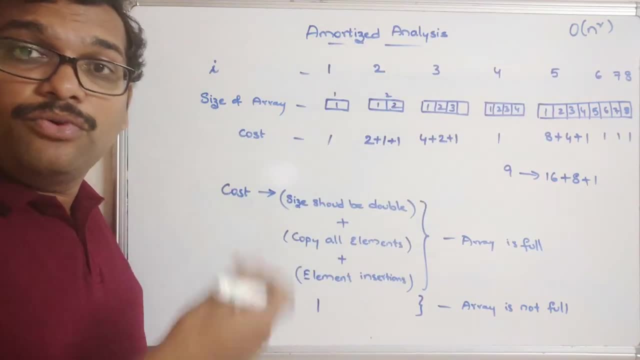 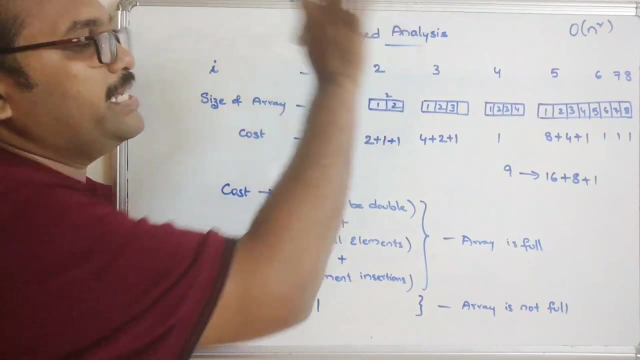 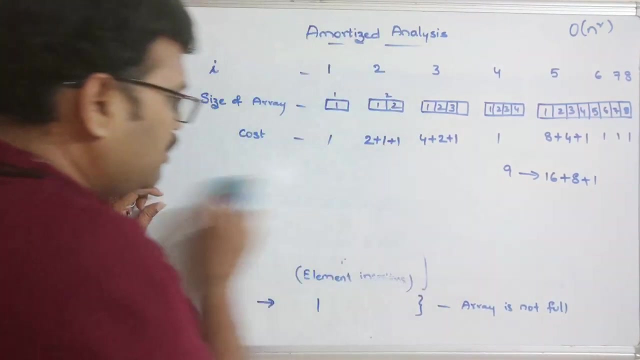 okay, so different operations, all are the different operations. so we have to apply, uh, the same thing for n elements and we have to take the average. because of this amortized analysis, this is the average performance of an algorithm. now let us consider: so we have find the cost of all the operations, and this will be keeps on moving. 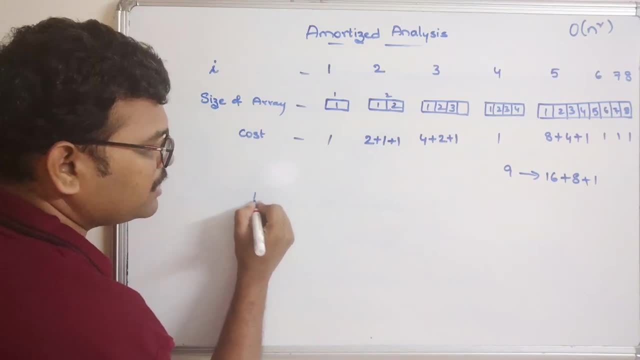 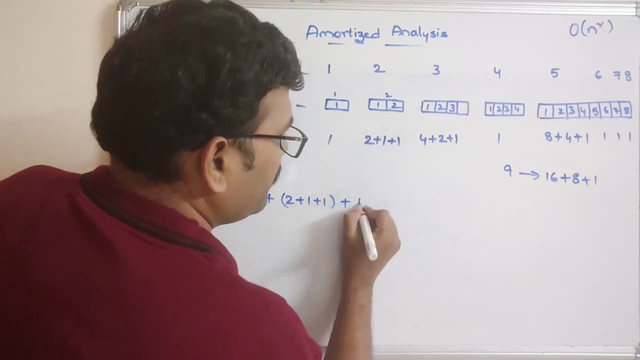 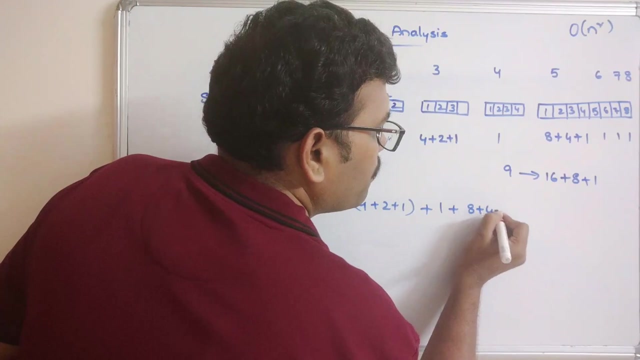 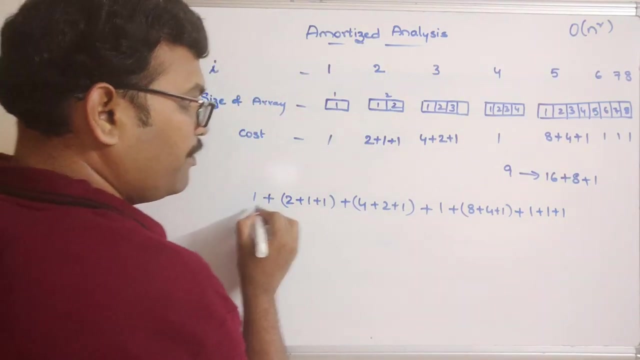 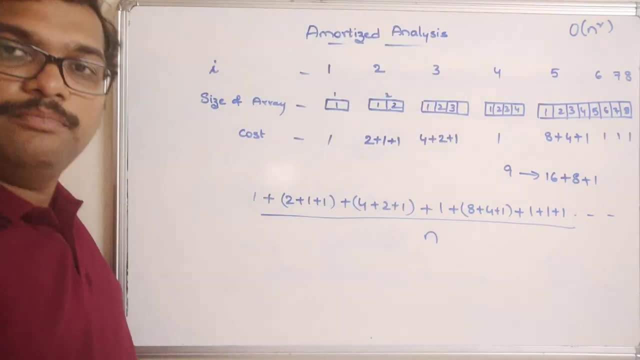 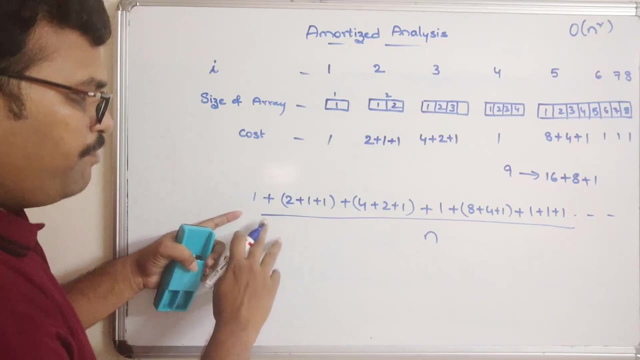 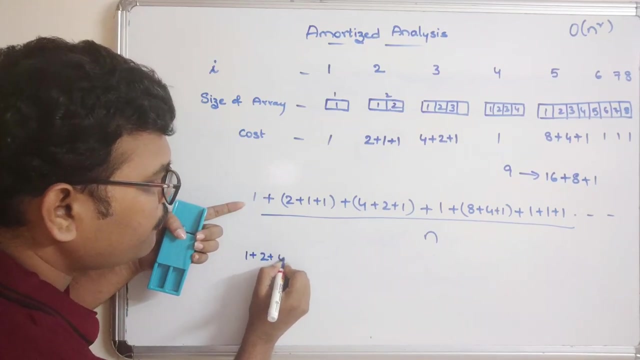 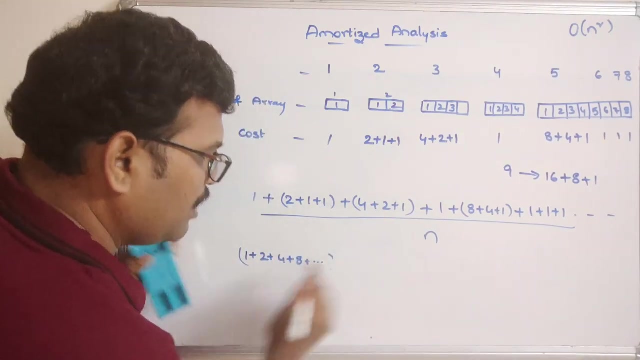 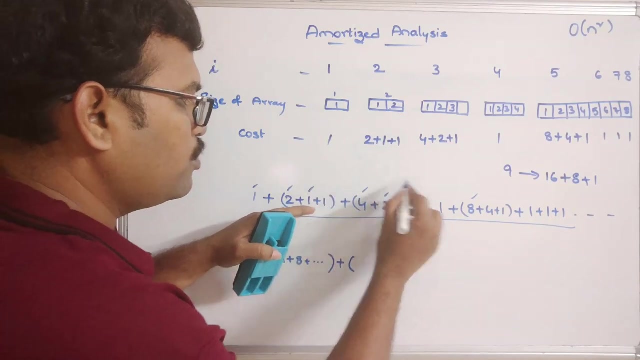 some moving and divided by n because we have to average. so these are all the cost of n operations. so you can observe, we can replace this with: okay, we can replace this with: so 1 plus 2 plus 4 plus 8 plus and so on, and similarly plus, plus, see 1, 2, 4, 8. again 1 2, 4. 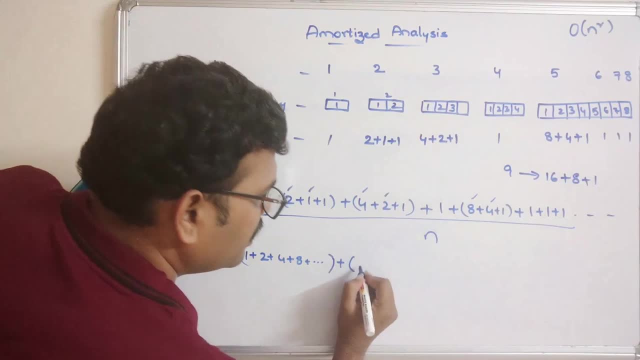 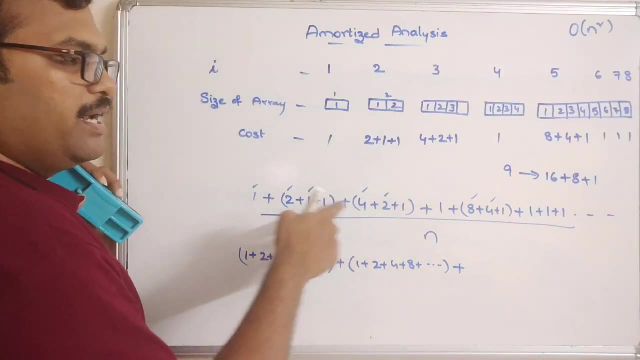 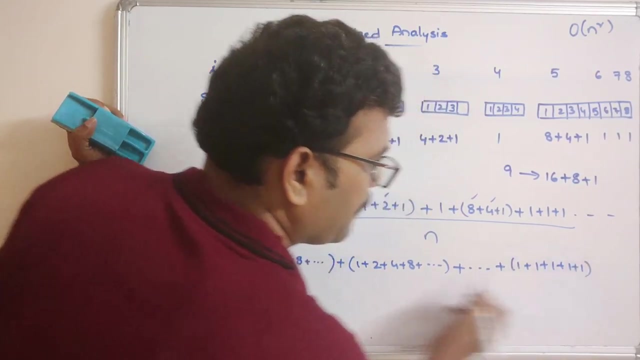 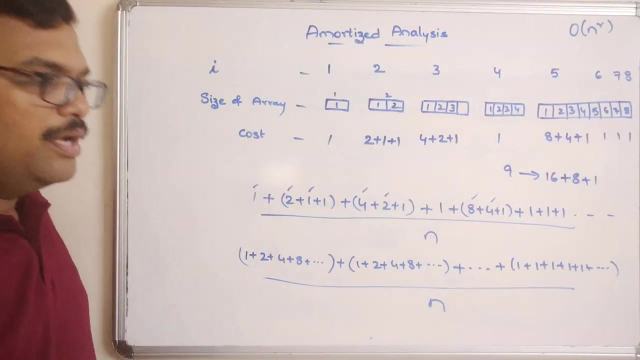 and so on, and again we will get 8 here right. so I get 1 plus 2 plus 4 plus 8 plus, and so on, plus. finally we will get all ones right, and so on, plus, we will get all ones or ones divided by n. so this is also keeps on going, okay, so we will get. 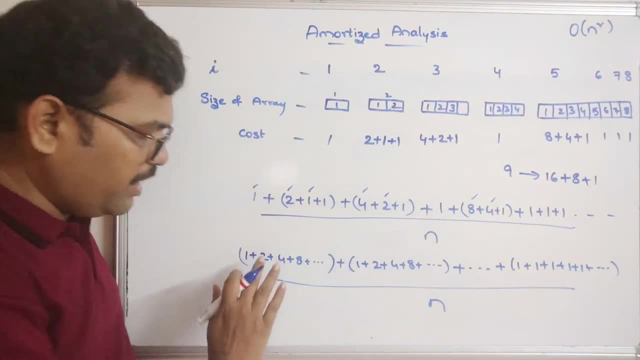 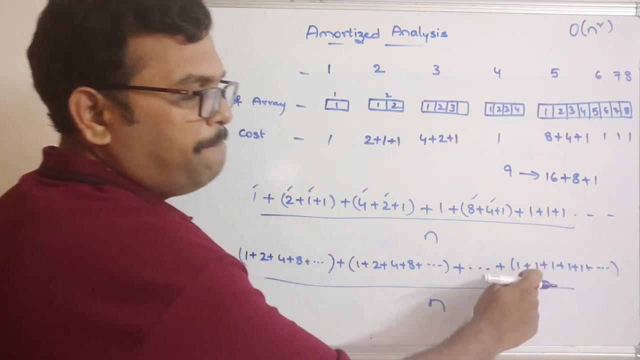 only these time these type of iterations. so we get 1 plus 2 plus 4 plus 8, again 1 plus 2 plus 4 plus 8, again 1 plus 2 plus 4 plus 8, again 7, all once we can write like this. so we know the complexity for this particular. 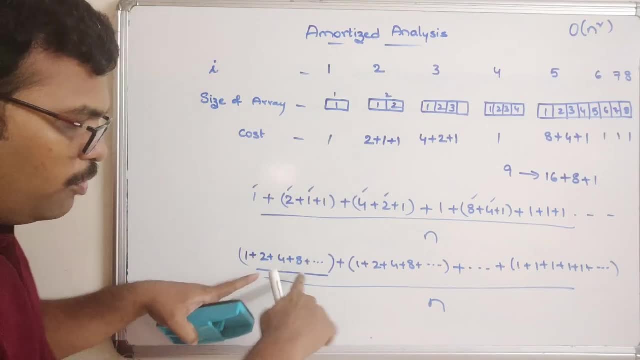 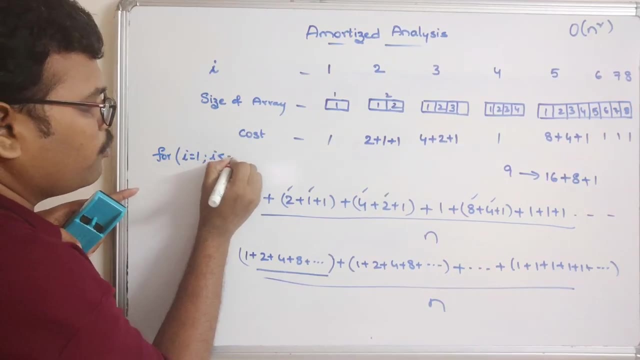 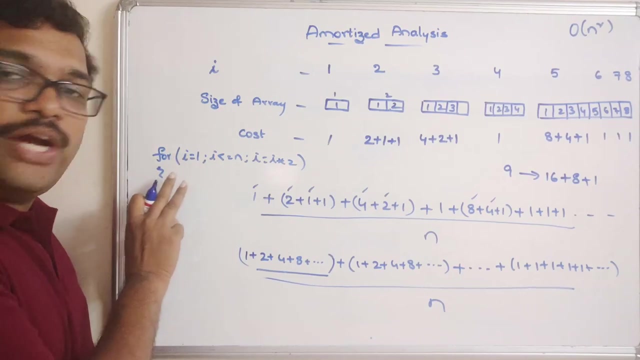 series. okay, see, if you want to get like this, simply you can analyze: i is equal to 1, i less than, or equal to n. i is equal to i into 2, so we have already seen such a time complexity, so which will be incremented with the two two times. so 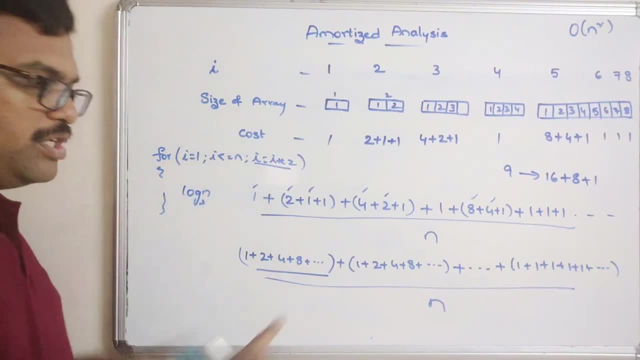 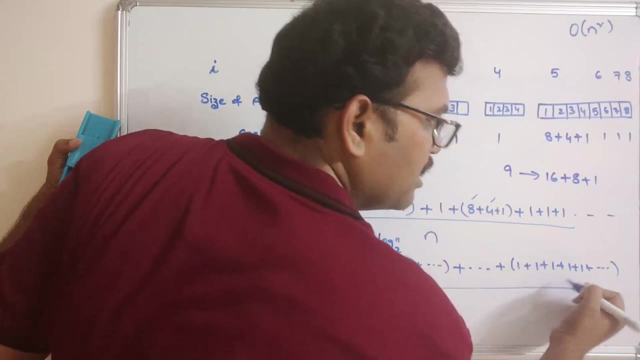 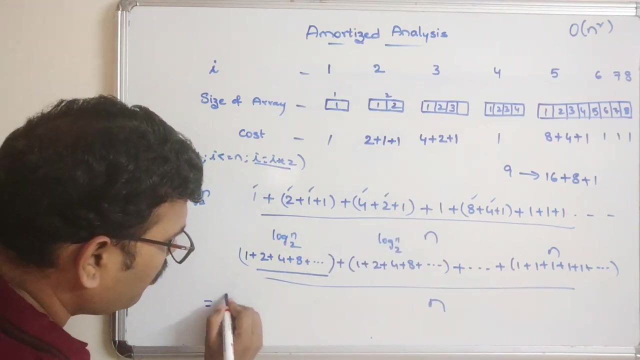 that we call it as a log n base 2, so simply we can replace this with log n base 2 and this is also log n base 2, and this is total n terms, so n times 1 will be added, so n terms. so what we can write here. order of log n base 2 plus. order of log n base 2 plus. 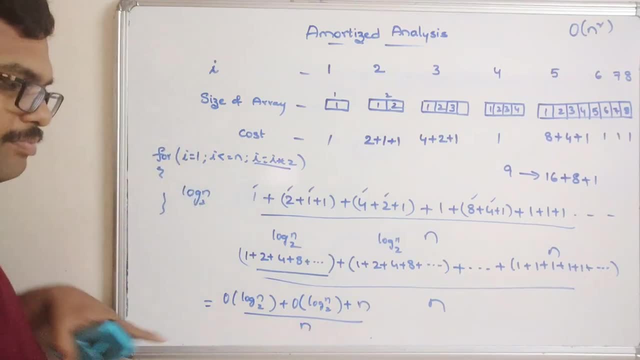 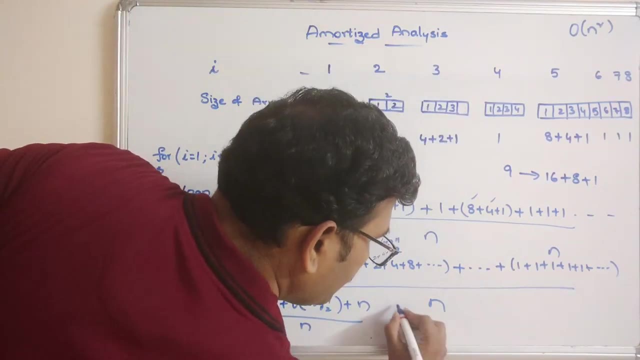 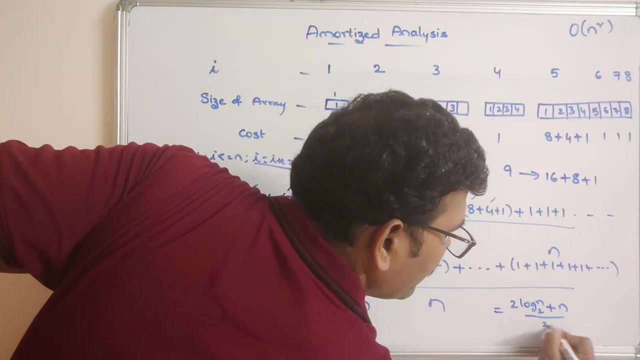 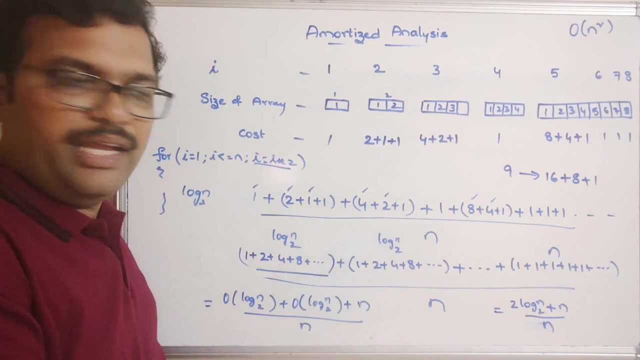 n divided by n. so what happens here? 2 log n base 2. so this becomes 2 log n base 2 plus n divided by 2, sorry, divided by n. so you can see we have to consider the highest degree. so among log n and n, which will be having the highest degree if we are having some function. 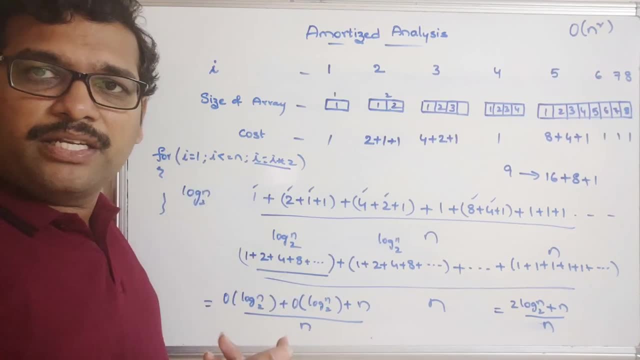 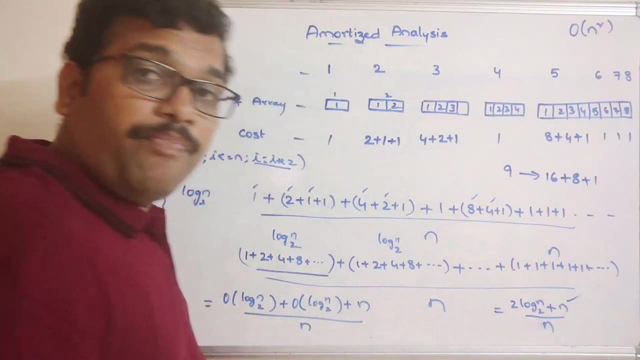 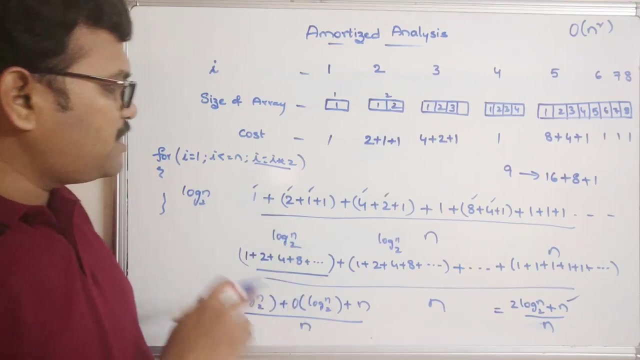 and we are trying to calculate the time complexity. we have to find out the highest degree. so what is the highest degree in this equation? so n according to the growth rate. so just visit our previous sessions so that you will be understanding how we got this log. n and. 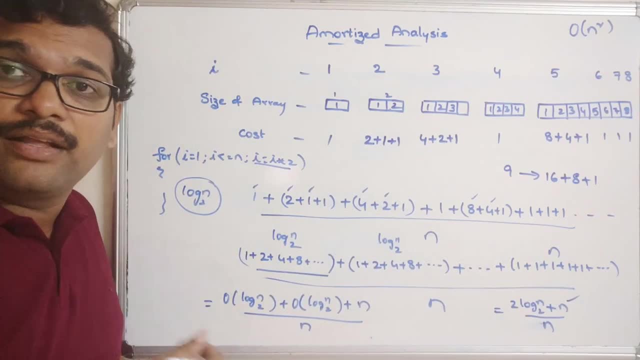 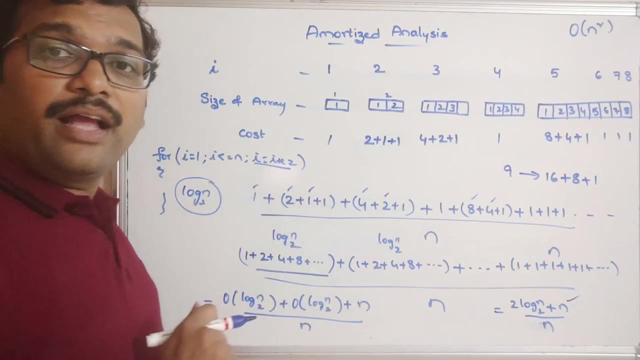 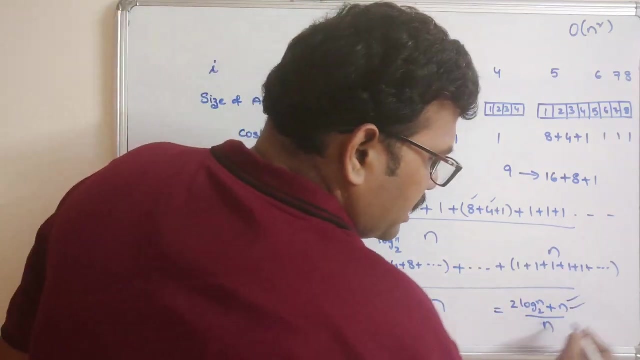 how we are selecting this? n right, so finding, calculating the time, complexities and the growth rate. so these two sessions you just go through so that you will be getting the clarity about that one. so I will share the complete playlist in the description box. okay, right, so we have to consider this one and this will becomes and this will becomes order. 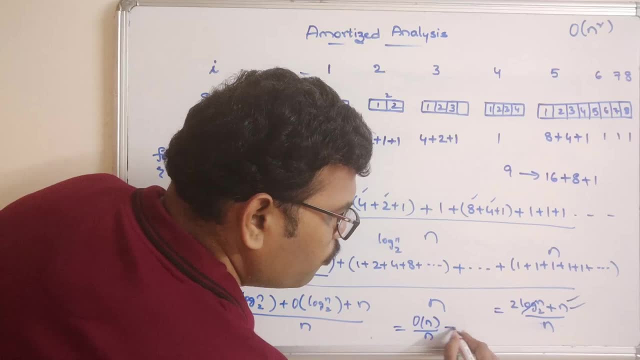 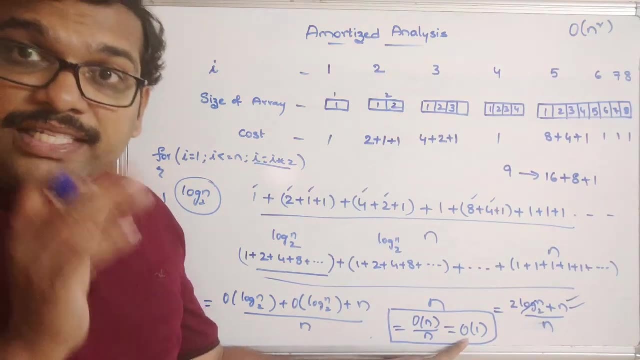 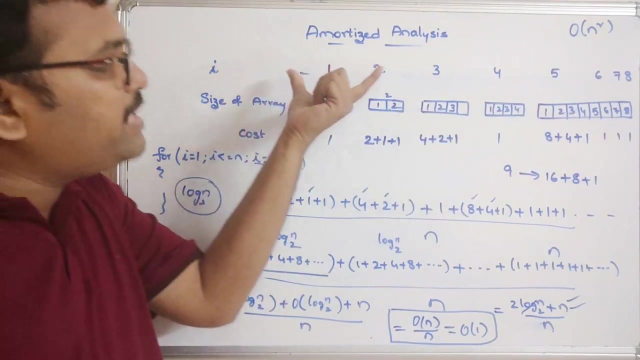 of n divided by n, which is nothing but order of 1, see order of 1. so the same problem, what is the worst case, time complexity is the order of n square. and if you are using this amortized analysis, particularly the aggregate method, so this amortized analysis is also having. 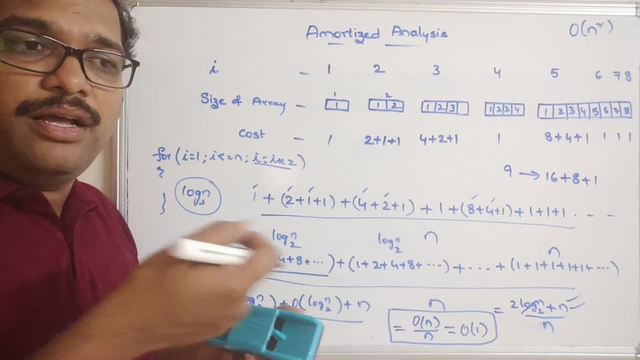 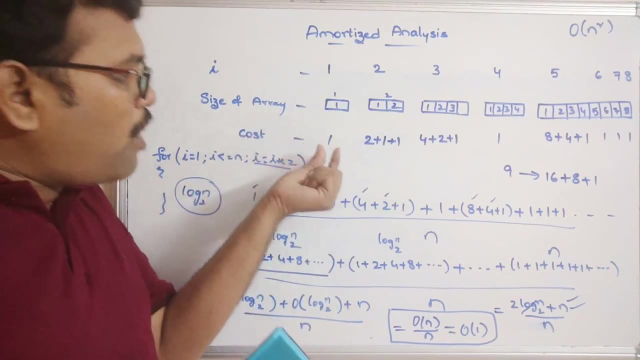 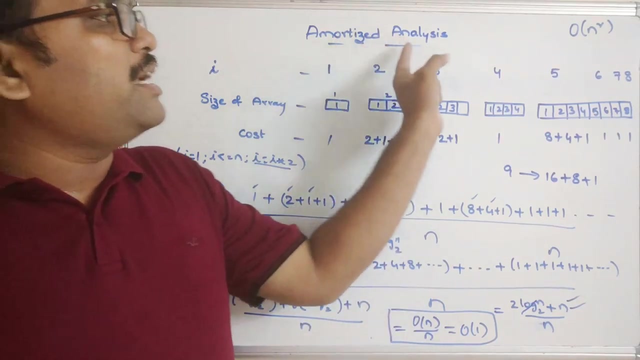 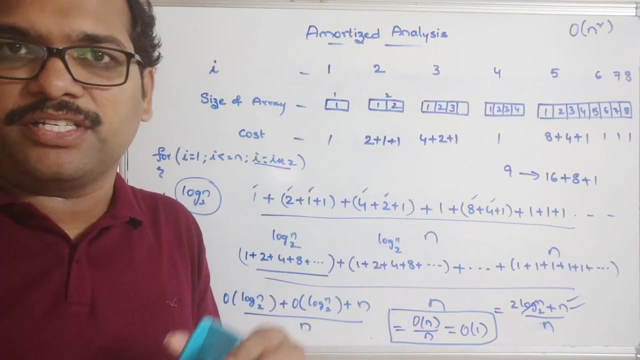 a different methods, right, so counting method, then aggregate method, potential method- right, so this is an aggregate method. so here we have to calculate the cost of each and every operation and then we have to perform the average so that we will get the amortized time complexity which we call it, as a average performance of an algorithm over a set of operations. so 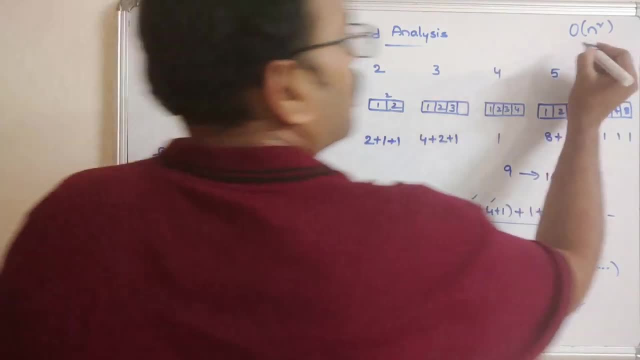 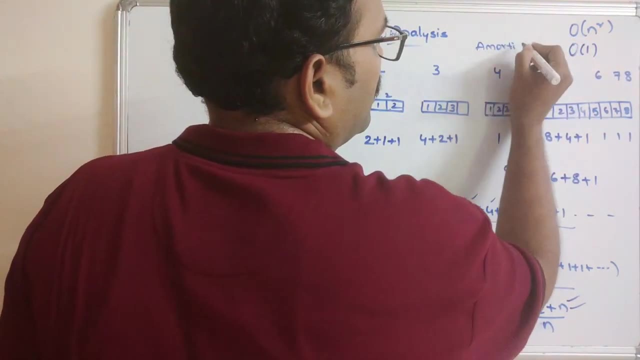 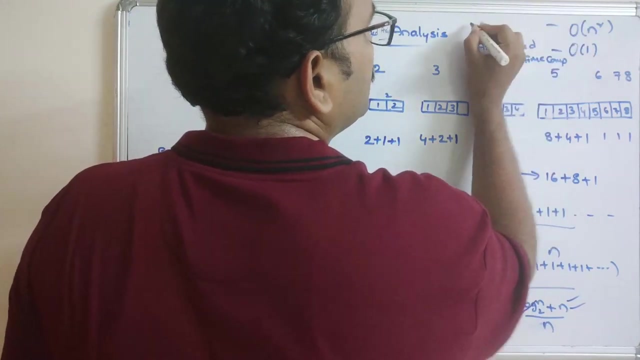 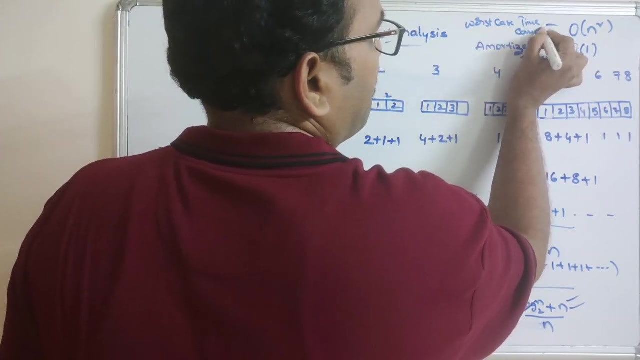 that is the most important. okay, so order of n and this is order of 1. this is amortized time complexity, amortized time complexity, and this is a worst case time complexity, worst case time complexity. right, so there you can find the difference. so, worst case time complexity. 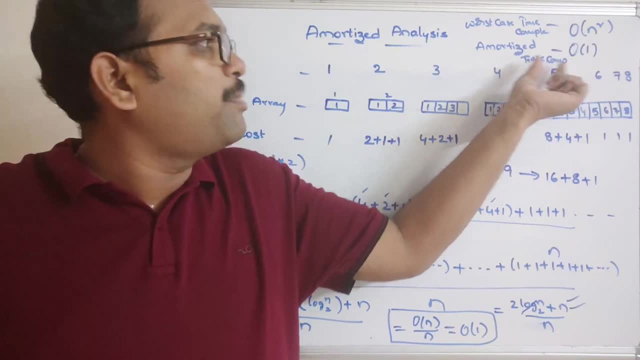 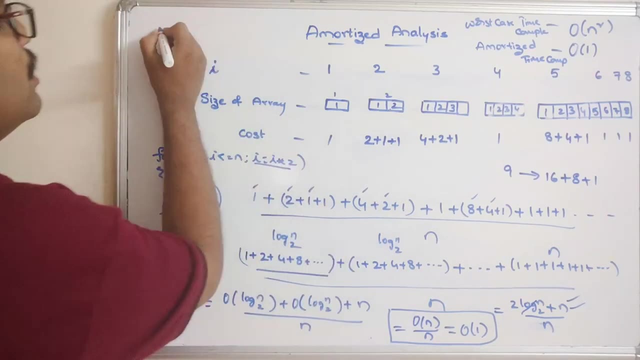 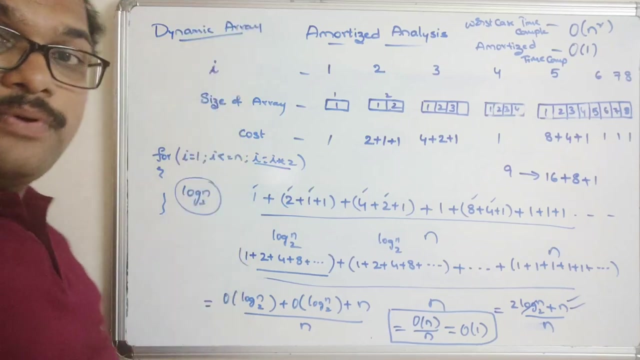 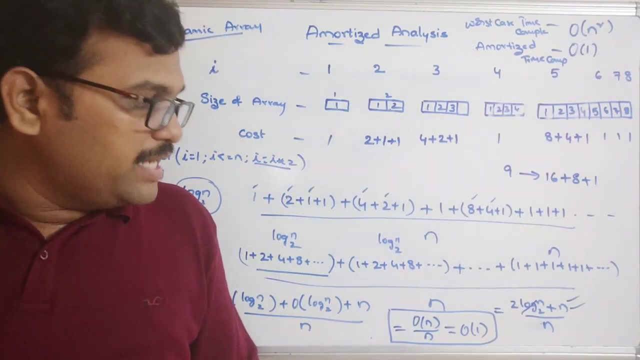 of order of n square and where amortized time complexity will be the order of n inserting an element into an dynamic array. so this problem is for inserting an element into a dynamic array. so previously we are having some order of n square. so in our previous example we 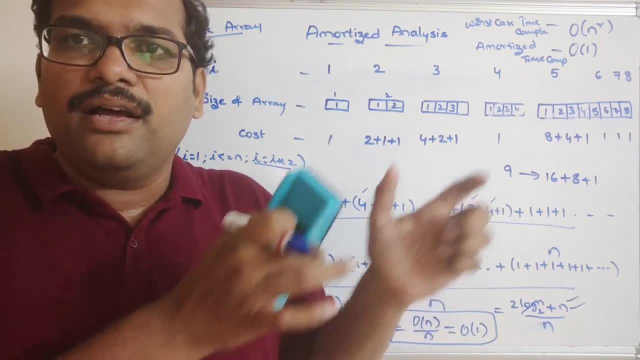 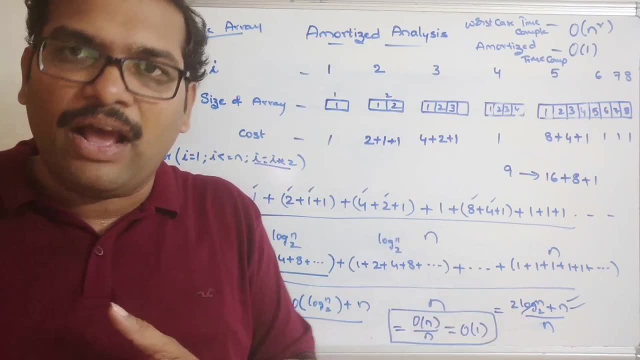 have seen. so if a person needs some monthly expense of 10 to 15 thousand, so we will be able to calculate this. this is a very interesting example and we will be able to calculate the expenses to run a family, so how much he requires to run a family on an average. we have. we have.